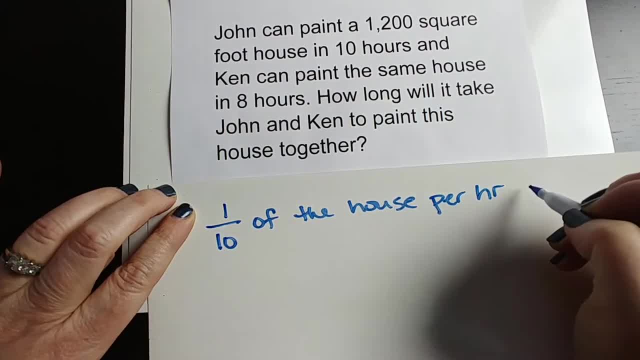 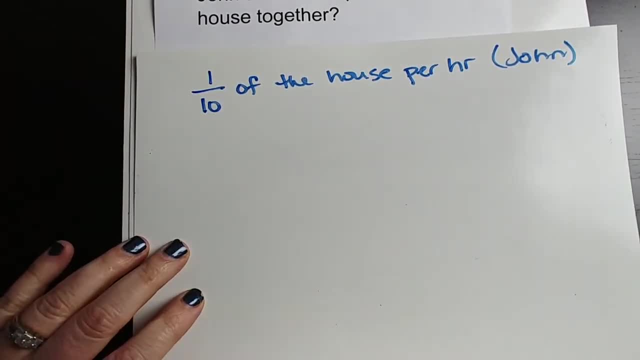 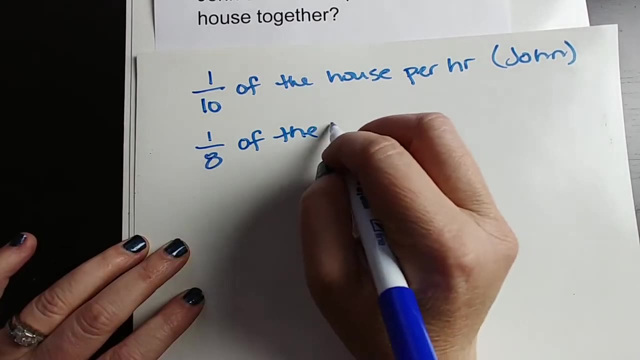 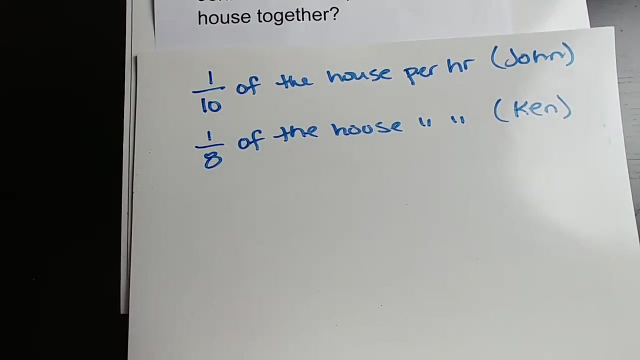 that's how much work he does per hour, Probably say that this is John Okay, and if Ken can paint the same house in eight hours, then Ken can do one-eighth of the house per hour And that's Ken Okay. so then it's easy to see and we 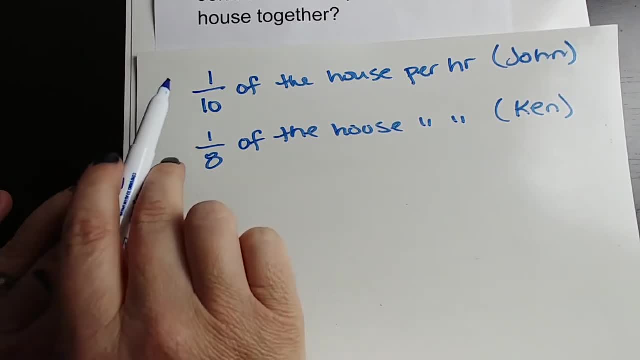 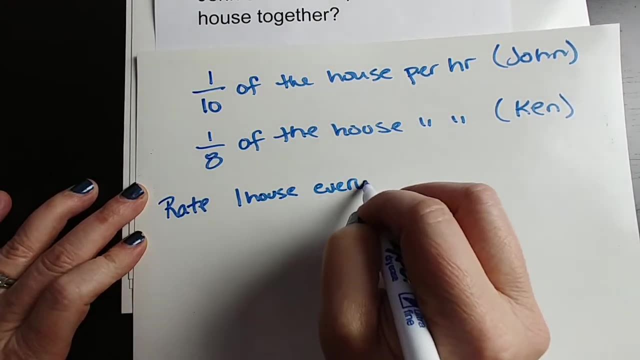 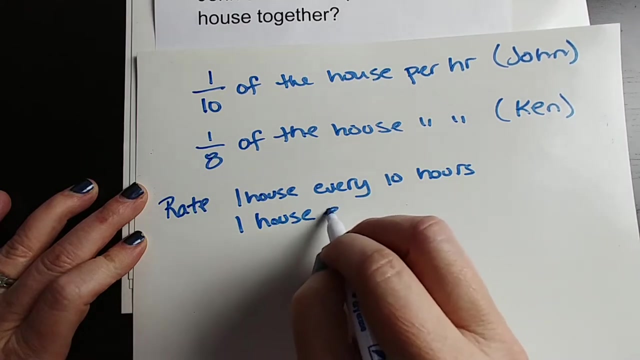 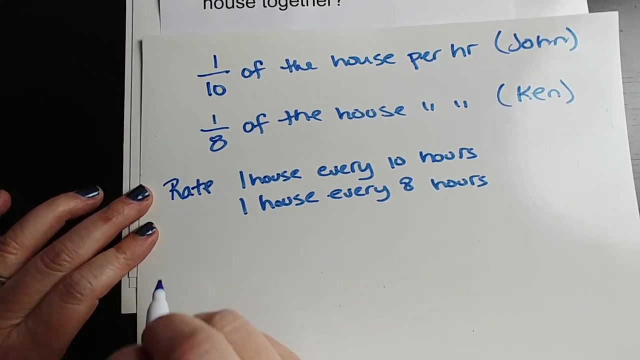 can read this as: one house per 10 hours, right, So he has it's a rate of. so the rate is one house every 10 hours, Okay, it's important to be able to see that. or one house every eight hours, Okay, because what we can say then is all right. well, so together their rate. whoops can't spell. oh, that's. 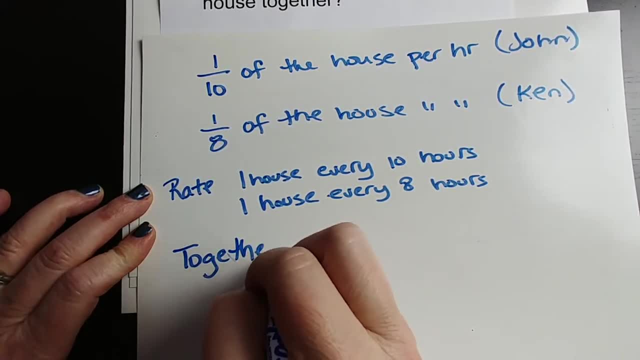 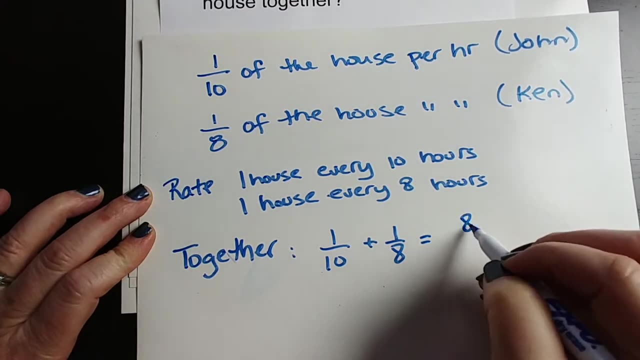 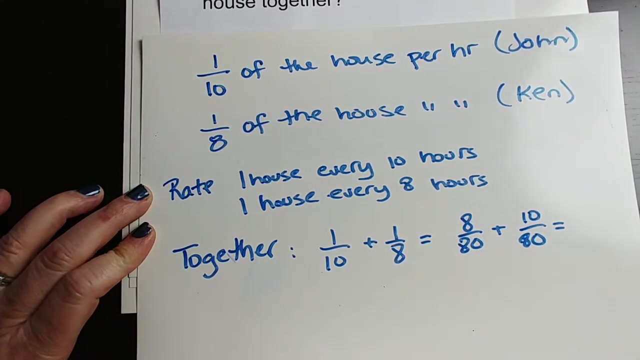 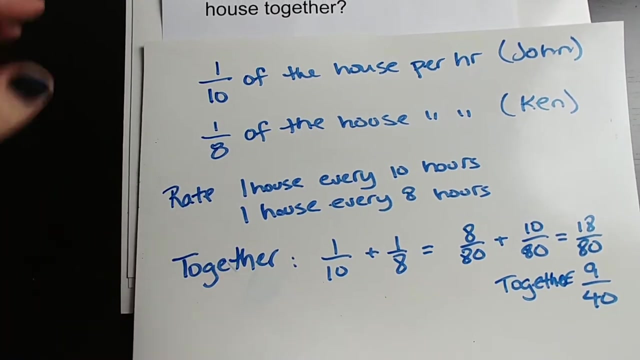 awful, I gotta fix that, really sorry. together their rate is one-tenth plus one-eighth, Okay, so that's basically eight um 80ths plus 10 80ths, right, and that is 18 80ths. Well, that's ugly. So nine 40ths, that's their rate together. So together, All right. so together, nine 40ths, All. 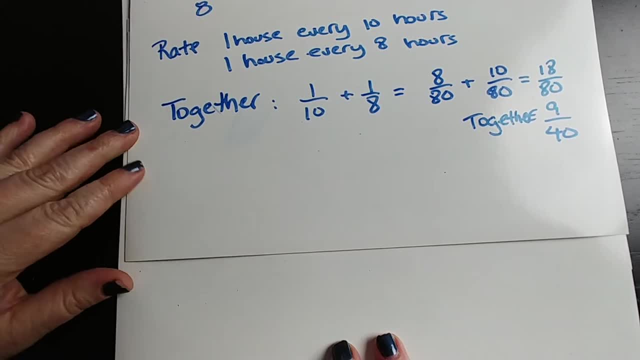 right, let's get me some more room here. So how do we turn this into the answer? It's actually quite easy. It's not like I'm really busted on this, but let's get back to number 40.. So if we know that, 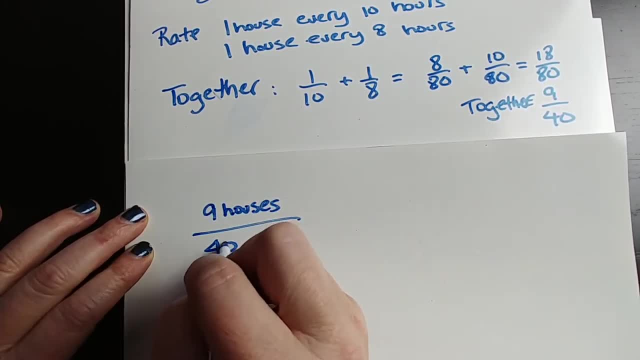 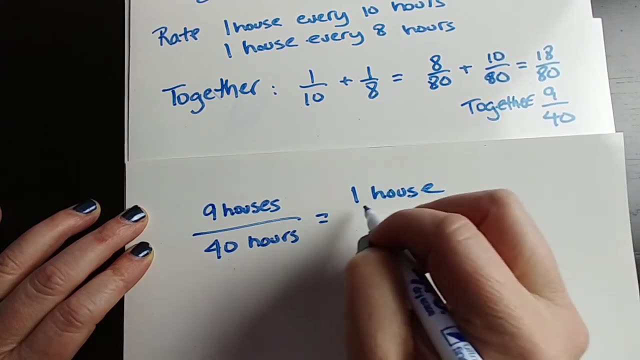 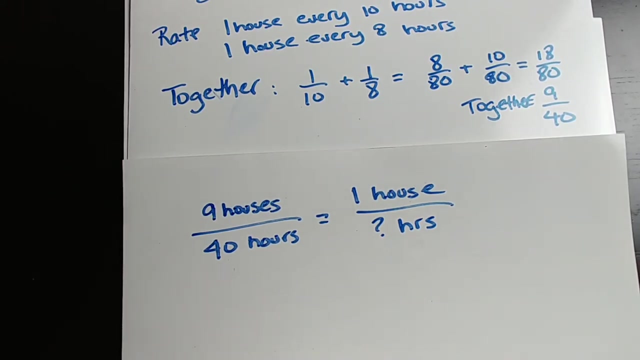 together they can do nine houses every 40 hours. I want to know how long for one house. So one House, question mark hours. That's it. that's all we have to do once we get their together rate of 940.. We set it, We make a proportion by setting it equal to 1 over A variable. So we're going to say 9 over 40 equals nine una In nine, 2.4 o Toma. Oh, that's a fairly simple answer. fortyths. So if we know that together they can do nine houses every 40 hours, I want to know how long for one house? so one house, So one house. Question mark. hours, That's it, that's. Oh, one hour hours, That's it. that'sulas Shakey, Oscar in methodicerezse up today. all cause shapes. 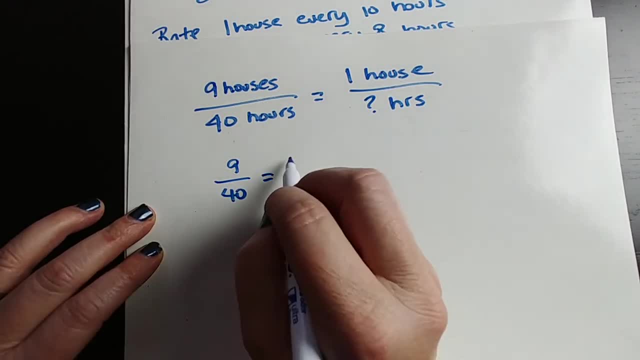 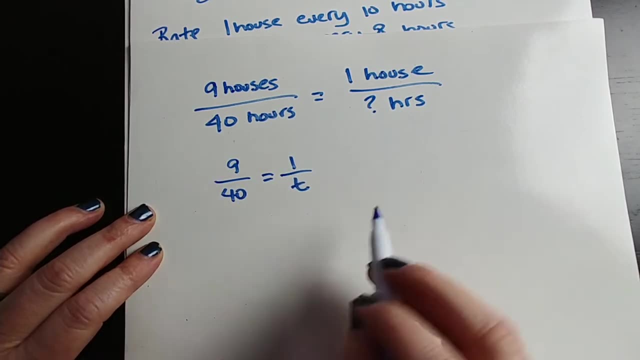 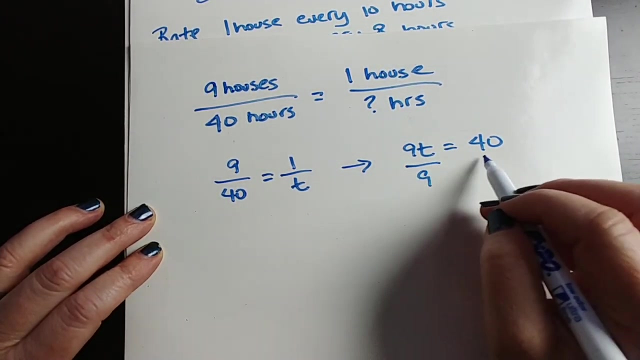 So we're going to say 9 over 40 equals 1 over t. Usually they make you do t for time. You know you can cross, multiply to solve a proportion fairly easily. So this turns into 9t equals 40.. Okay, we're going to divide by 9, divide by 9, t equals, or it's actually a repeating decimal. 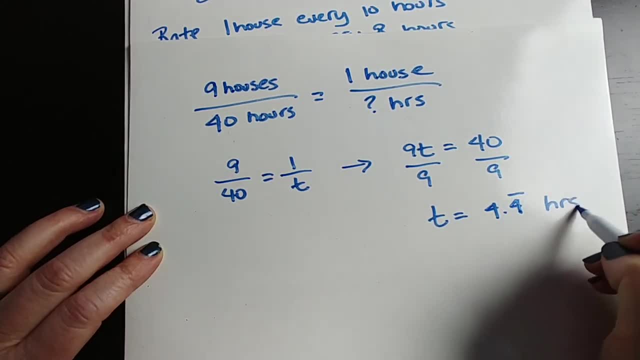 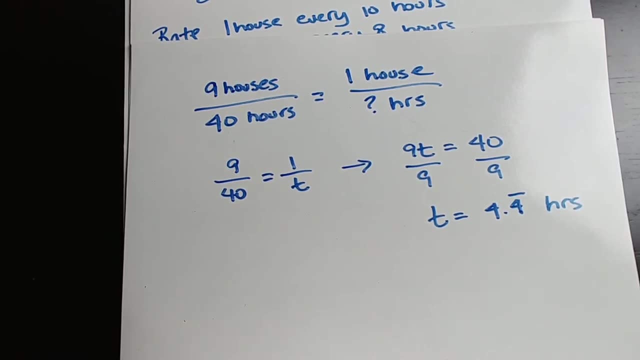 so 4.4 repeating hours, There you go. that's how long it would take them together. They're these horribly unrealistic problems that somehow show up in every algebra class we ever take. I hope this helped These get easier. you just have to set them up the same way each time. 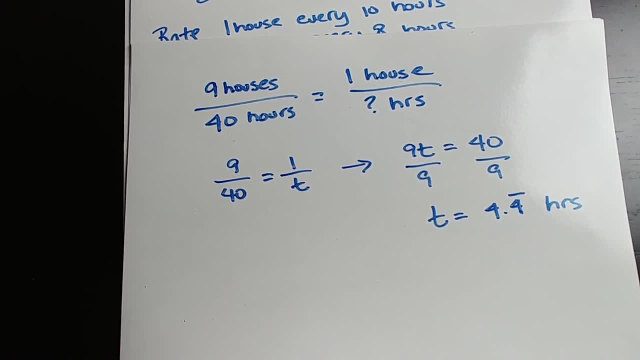 If you have any questions, pop them in the comments. Be sure to subscribe to our YouTube channel. that way I can do your problem next. 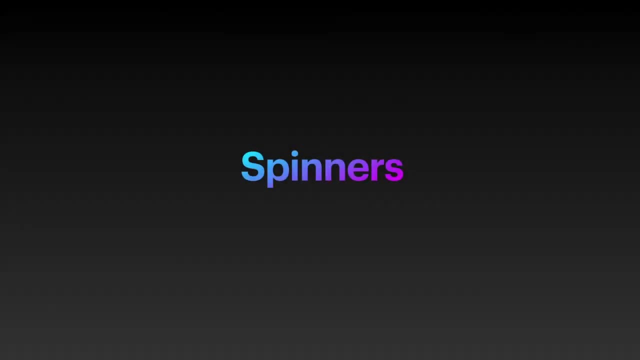 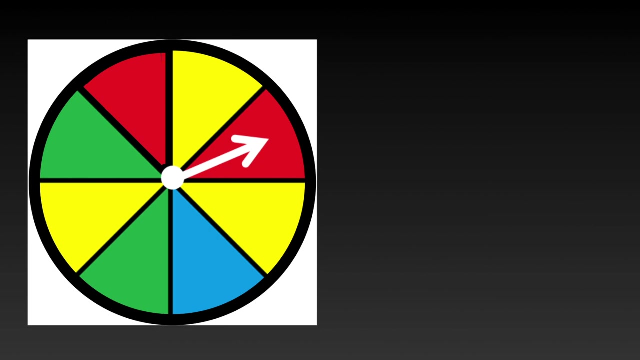 We are continuing our unit on probability today and we will be talking about spinners. Here is an example of a spinner. You may have seen a spinner before in a game or at a fair, and today we are going to analyze the spinner using probability words and remember, analyze means to look closely. 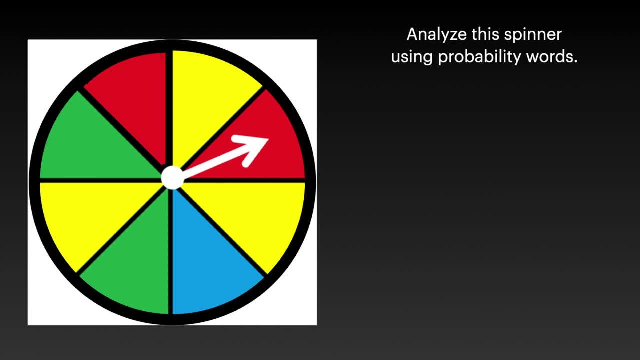 So we're going to look closely at the spinner and we're going to use probability words. Just to remind you of the probability words that we've talked about so far, this unit- we will be using the words certain, likely, equally likely, unlikely and impossible. 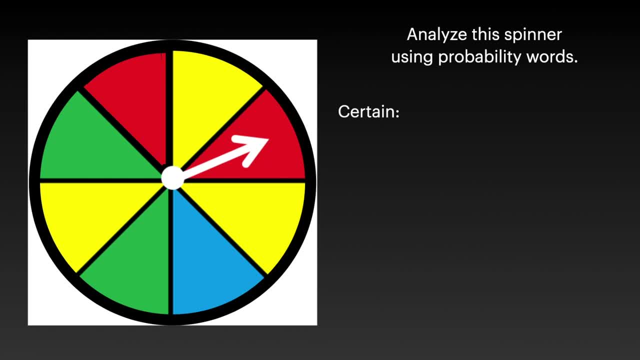 Let's start with the word certain. Which color am I certain to land on? Well, if I were to spin this spinner, I could land on red, yellow, green or blue. I'm not actually certain. I'm not certain to land on any specific color, So no color is certain, since there is more. 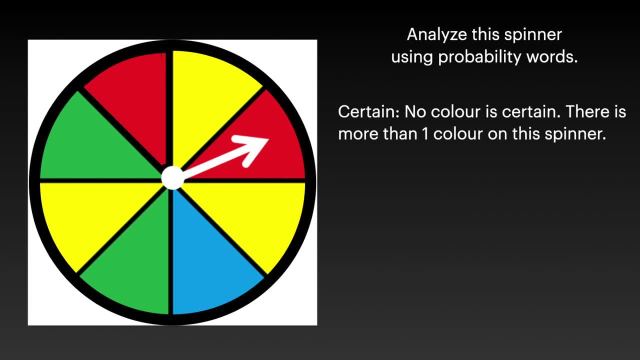 than one color on this spinner. If the spinner was just one color, then I would be certain to land on that color. Let's move on to likely now. if I were to spin this spinner, which color would I be most likely to land on? I can answer this question.